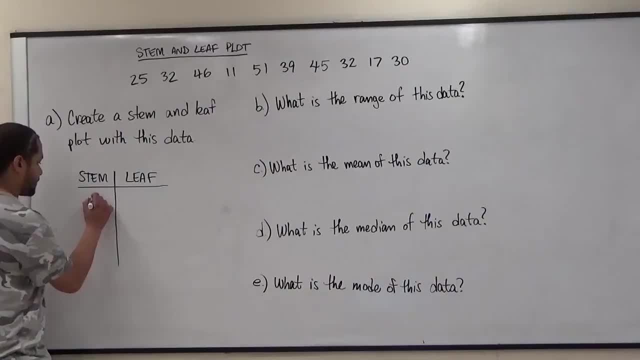 fifties. So we should have five stems here. So we have a ten, we have a twenty, we have a thirty, we have a forty and we have a fifty. Now, if your data goes beyond some value- let's say we had a seventy in this and there were no sixties value- we'll still put in the six. 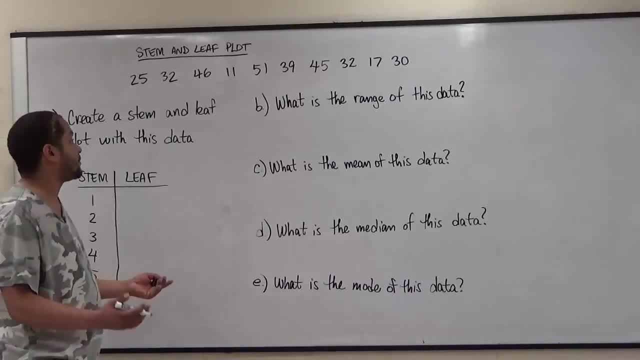 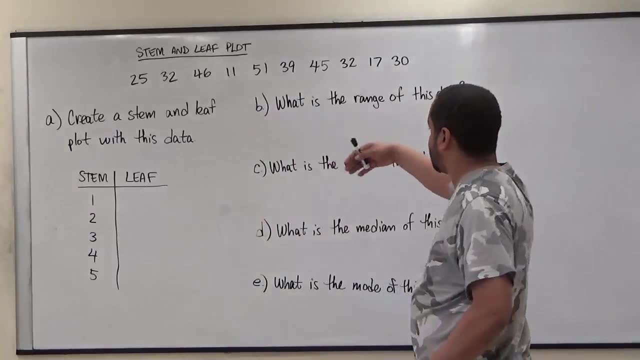 here and the seven and next to the six, there will be nothing because there's no sixties, or in the case of no seventies, there's no seventies, But in this case we have everything from ten to maybe like fifty-nine. So fifty, tens to fifties we have. so every 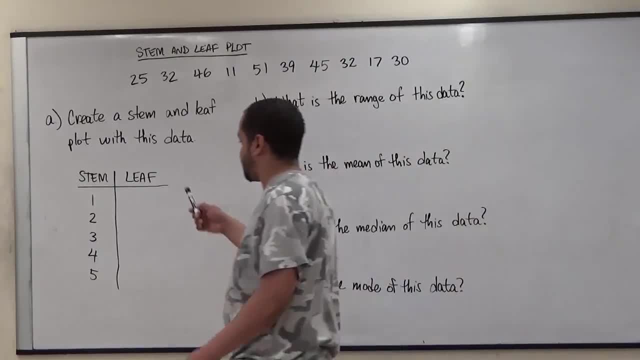 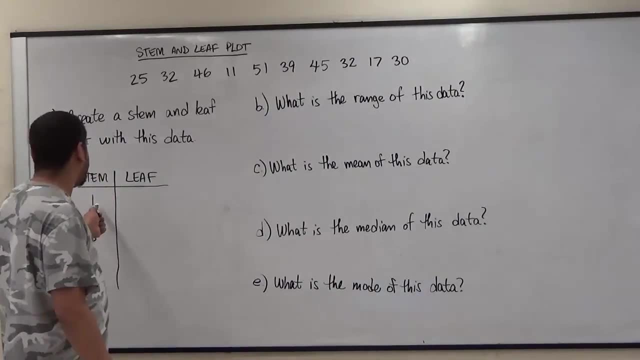 position here is going to have a leaf next to it, And it's fine. if the stem doesn't have a leaf, it would just remain empty. In this case, we don't have that situation happening. So now for the stems. we're going to start with the stem of ten and we're going to look. 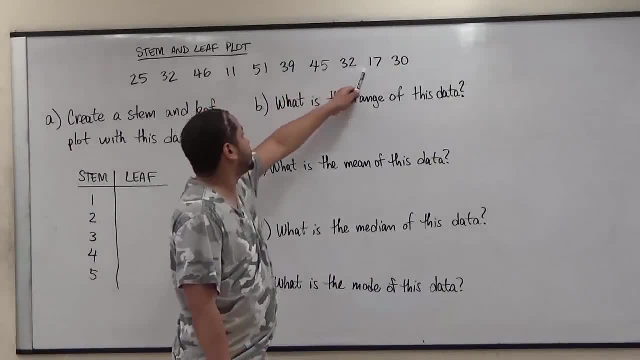 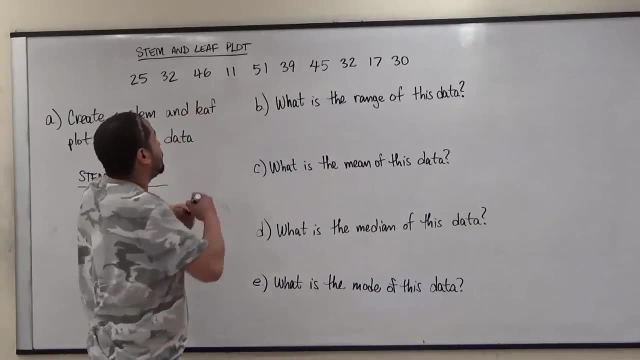 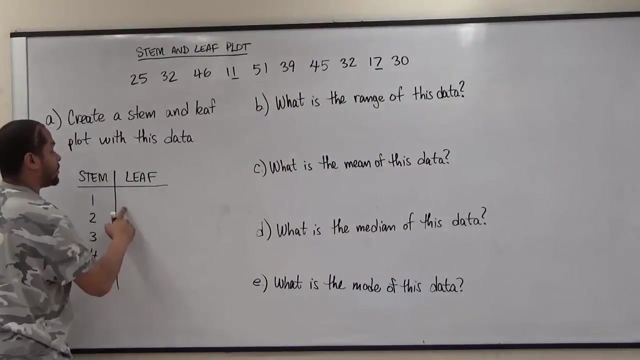 for how many numbers begin with one digit. So in our case we have eleven, we have seventeen and these have to be arranged in order. So our first leaf is going to be one and our second leaf is going to be seven, because they have the stem of ten and these have to go in order. 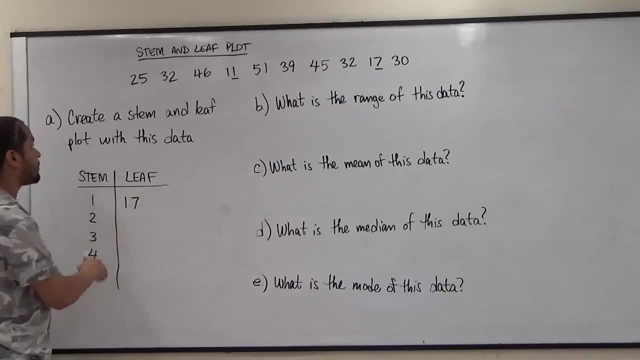 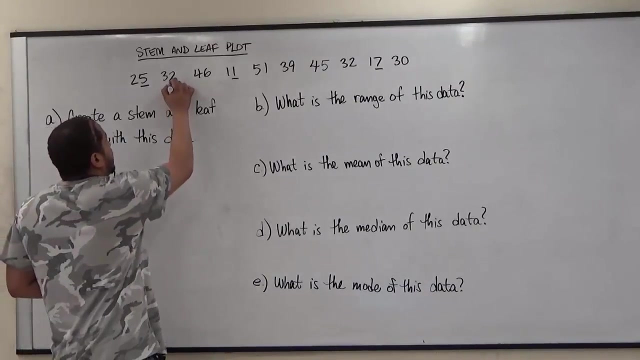 So we have one and seven for the leaves of one. For the leaves of two, we have just twenty-six, right, I mean twenty-five, the value of twenty-five, the leaf for twenty is going to be just the five. Then we have thirties. So now for thirty, we have a, two, we have nine, we have twenty. Great. One of them begins like this: The first before the last is served, And that means we have twenty-six for the last. So that means the number of leaves: we have twenty-six, we have twenty, twenty-aying. now for the fourth, we have ten, twenty- fourth. So now we can say whether or not we want. 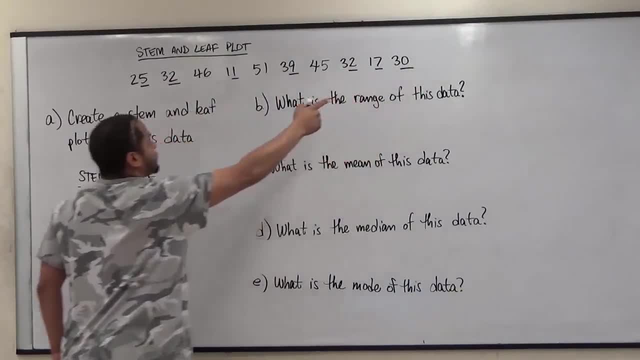 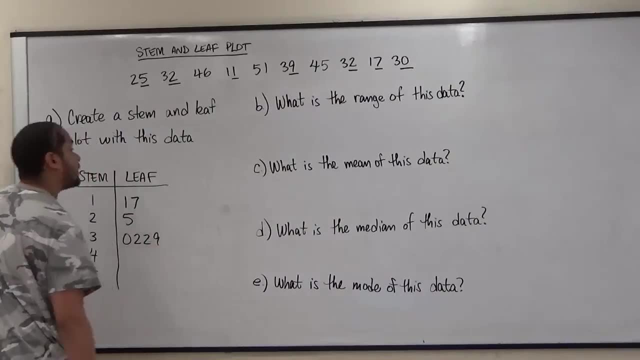 a 9,, we have another 2, and a 0. So we'll start with the 0,, followed by two 2s and then a 9.. We have 0,, 2,, 2,, 9.. Now for the 40s, we have a 6, and we also have a 5 here. 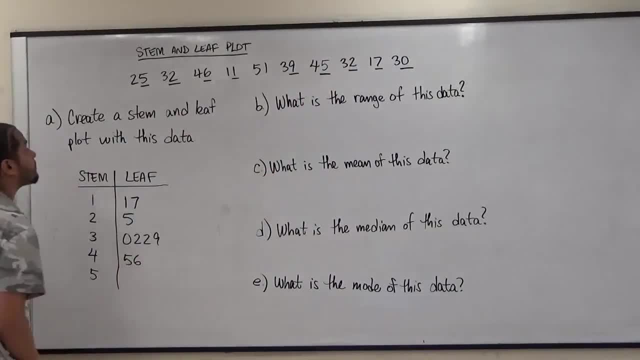 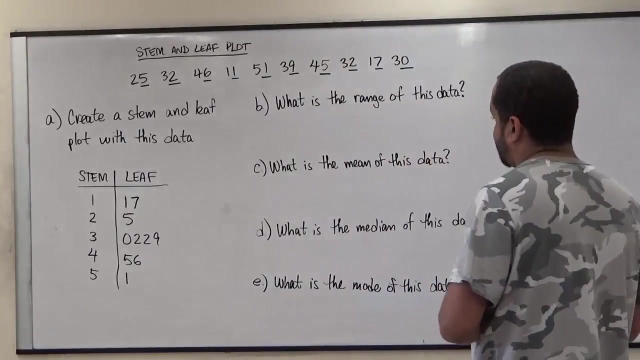 so we're going to put 5,, followed by a 6. And our last stem is 5, and for 5 we have just a 1.. This concludes the stem and leaf component of this video. After we finish this stem and leaf component, what we want to do then is find the range. So to find the range. 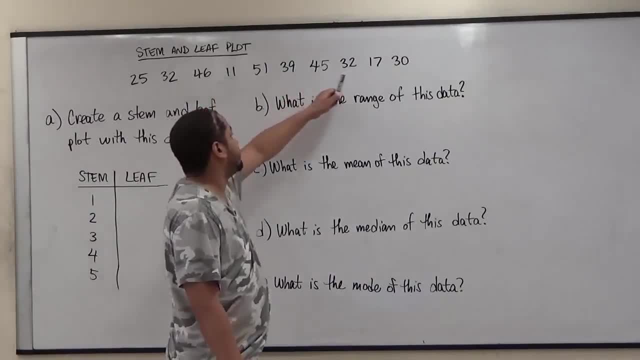 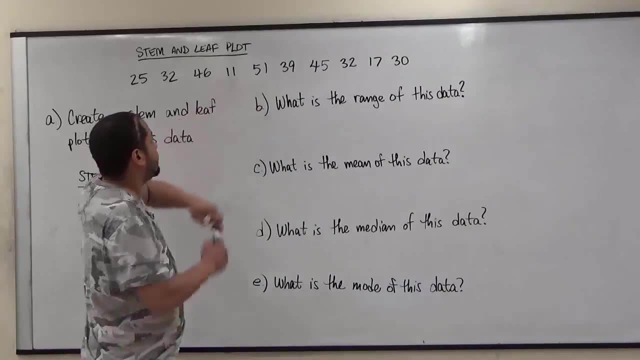 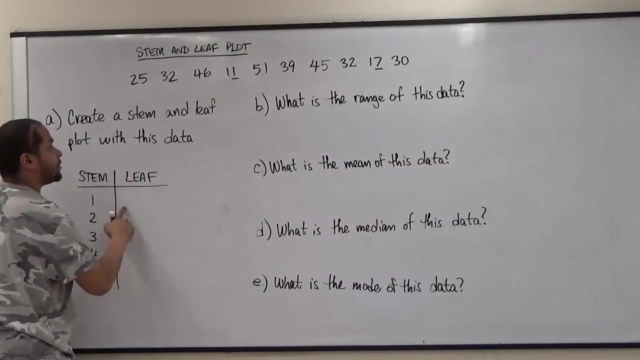 to look for how many numbers begin with one digit. So in our case we have eleven, we have seventeen and these have to be arranged in order. So our first leaf is going to be one and our second leaf is going to be seven, because they have the stem of ten and these have to go in order. So we have one and seven for 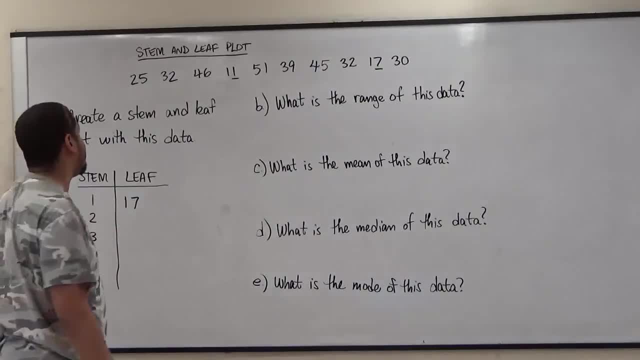 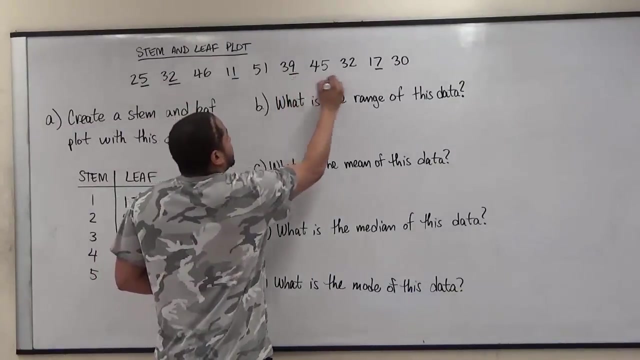 the leafs of one. For the leafs of two, we have just twenty-six, right, I mean twenty-five, The value of twenty-five, the leaf for twenty is going to be just a five. Then we have thirties. So now for thirty, we have a two, we have a nine, we have a ten, we have a fifteen, we 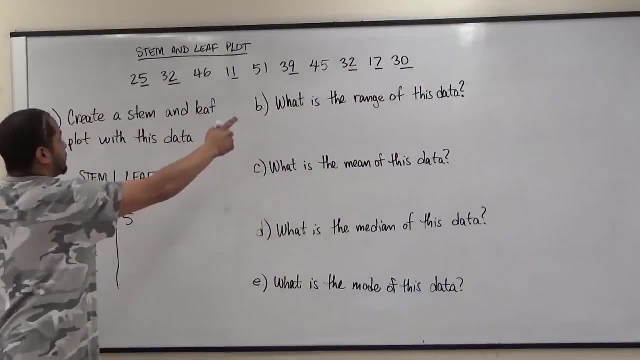 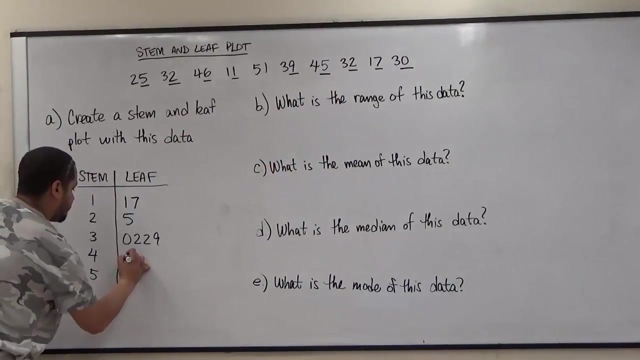 have another two and a zero. So we'll start with the zero, followed by two twos and then a nine. We have zero, two, two, nine. Now for the forties, we have a six and we also have a five here. so we're going to put five, followed by a six, And our last stem is five. 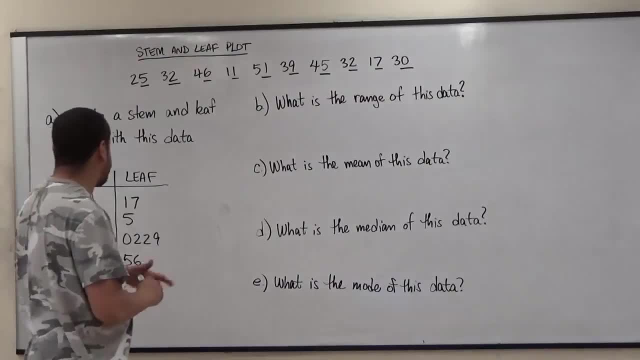 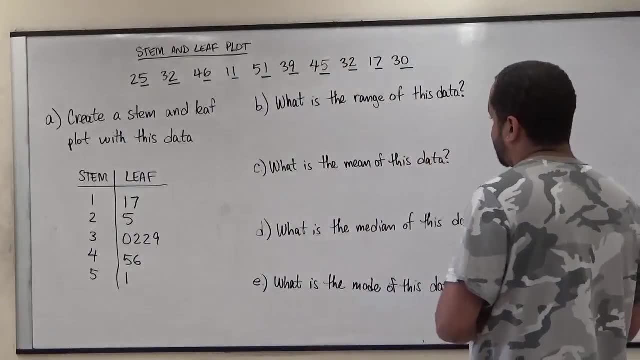 and for five we have just a one. This concludes the stem and leaf component of this video. After this stem and leaf component, what we want to do, then, is find the range. So to find the range, we take the first stem and leaf, and 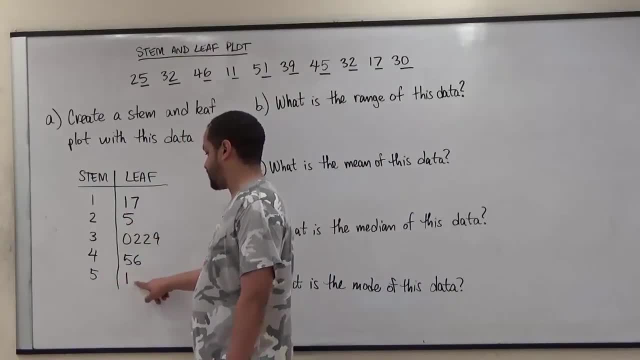 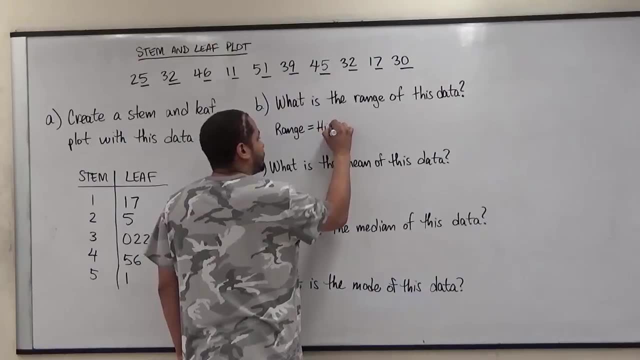 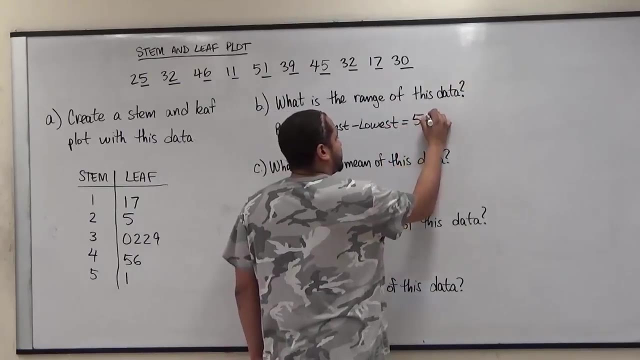 the last stem and leaf. So our first stem and leaf is 11.. Our last stem and leaf is 51. Now, remembering that the range is the highest value minus the lowest, our highest in this case would be 51. And we're subtracting 11.. 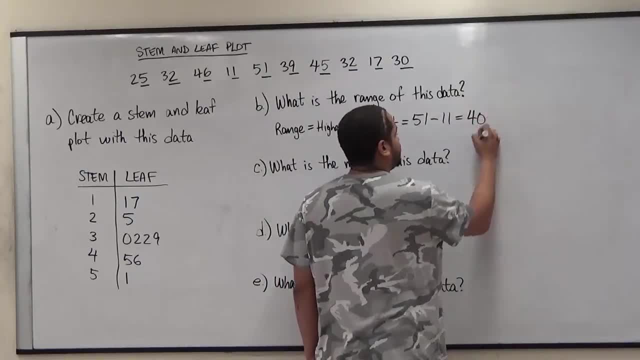 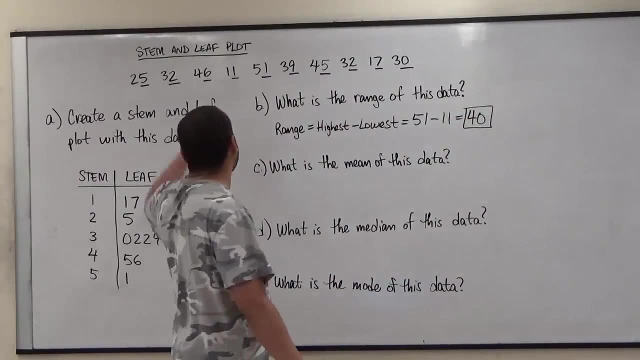 51. take away 11 gives us 40. So our range is 40.. Let's move on to the mean now. To find the mean, what we have to do is we have to sum all the values up right, And once we sum these values up, we're going to divide. 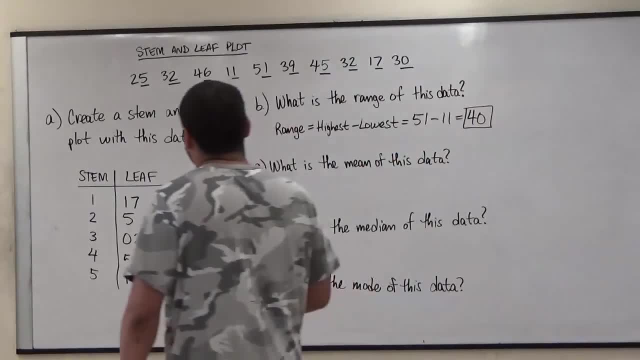 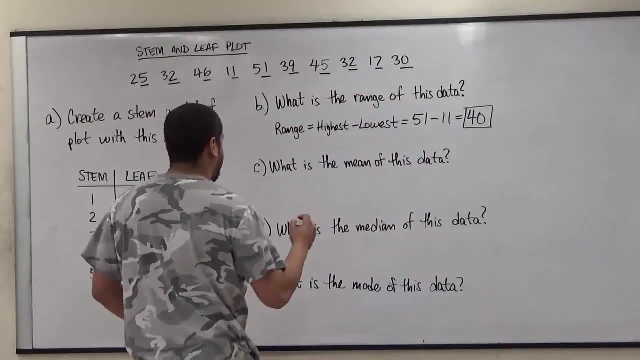 them by the amount of values we have. And here we see on this chart we have 1,, 2,, 3,, 4,, 5,, 6,, 7,, 8,, 9, and 10 values. So to get the mean, what we have to do to find x bar is: 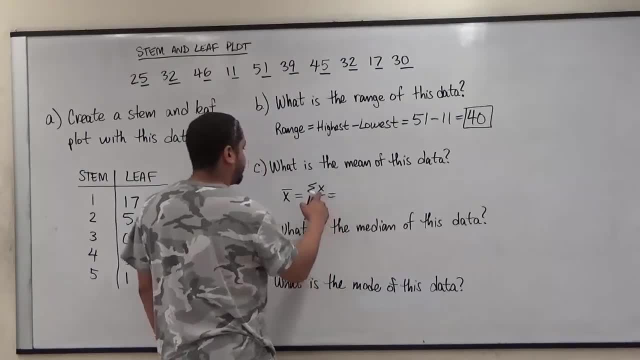 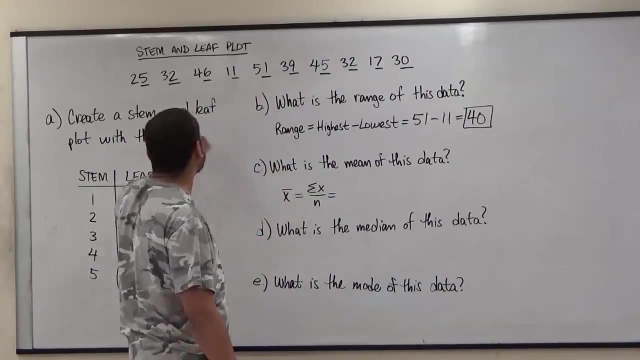 take the sum of every value and divide it by the n, Now the sum of x. what it represents is that x is every single sample value And this represents the sum of those samples. So we're just going to go ahead and add them up on the 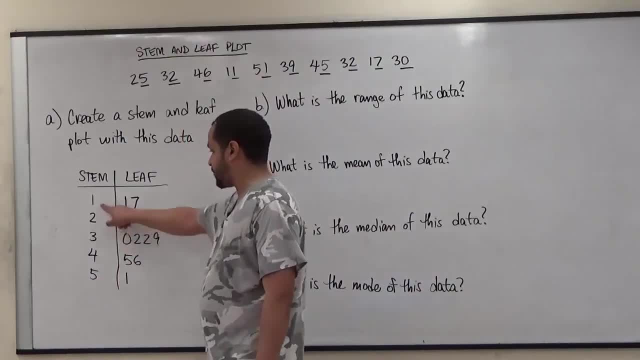 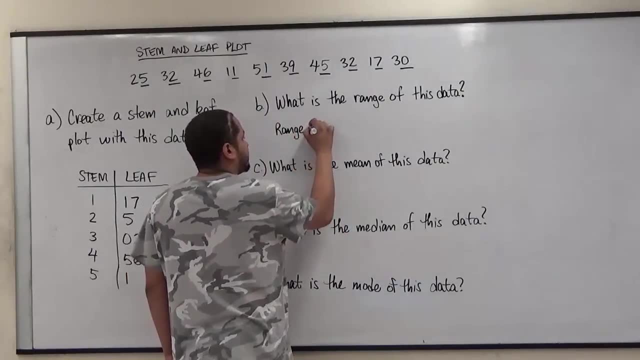 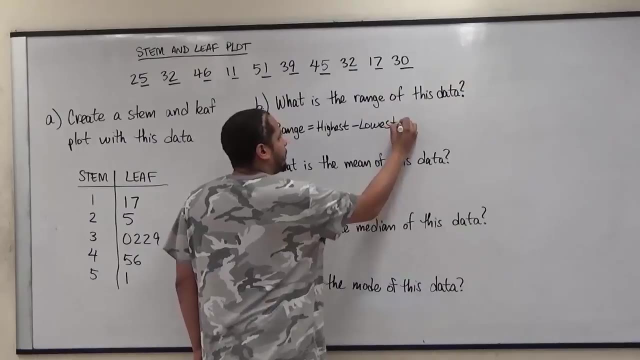 we take the first stem and leaf and the last stem and leaf. So our first stem and leaf is 11,. our last stem and leaf is 51.. Now, remembering that the range is the highest value minus the lowest, Our highest in this case would be 51.. 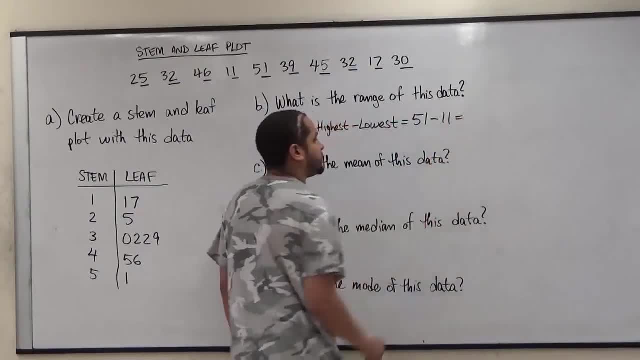 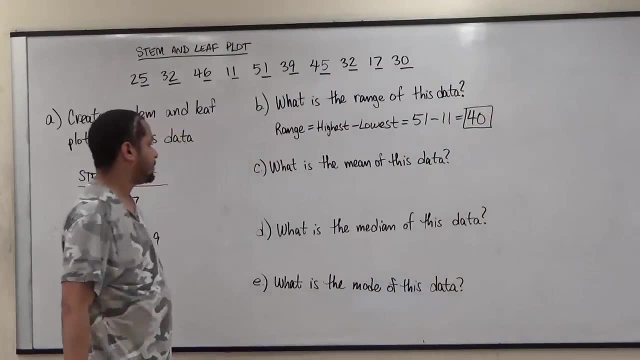 51, and we're subtracting 11.. 51 take away 11 gives us 40. So our range is 40.. Let's move on to the mean now. To find the mean, what we have to do is we have to sum all the. 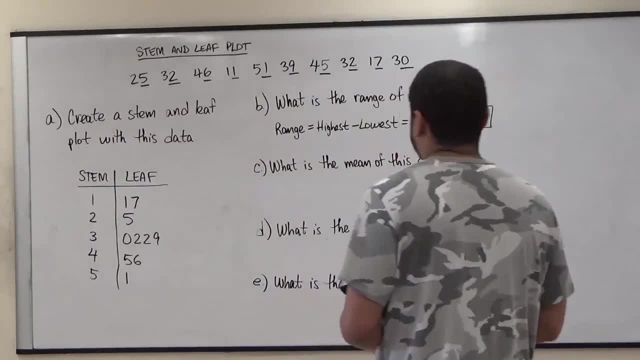 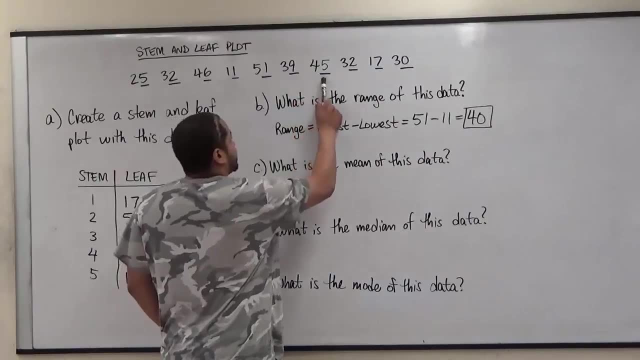 values up, right, And once we sum these values up, we're going to divide them by the amount of values we have. And here we see on this chart, we have 1,, 2,, 3,, 4,, 5,, 6,, 7,, 8,, 9, and. 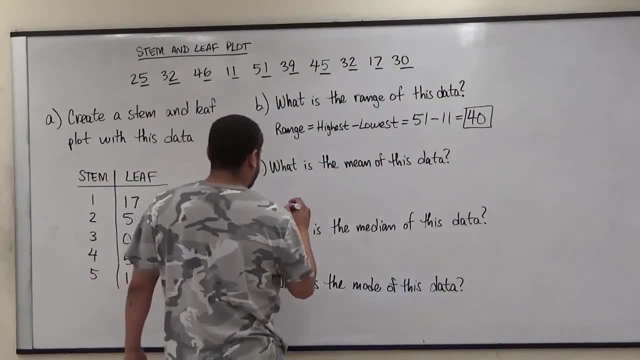 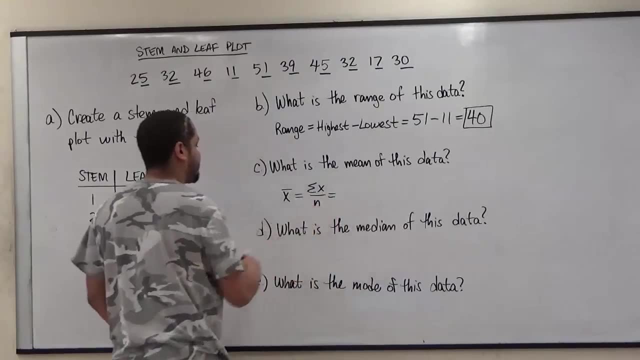 10 values. So to get the mean, what we have to do To find x-bar is take the sum of every value and divide it by the n, Now the sum of x. what it represents is that x is every single sample value and this represents the sum. 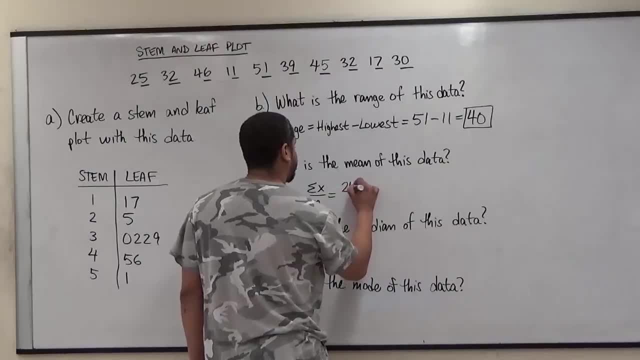 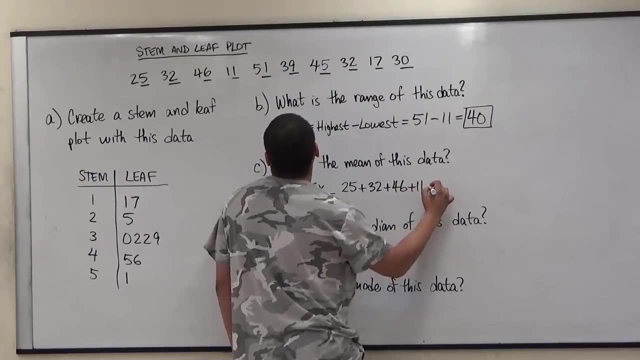 of those samples. So we're just going to go ahead and add them up on the numerator. So we have 25 plus 32 plus 46 plus 11 plus 51 plus 39 plus 45 plus 40.. So we're going to. 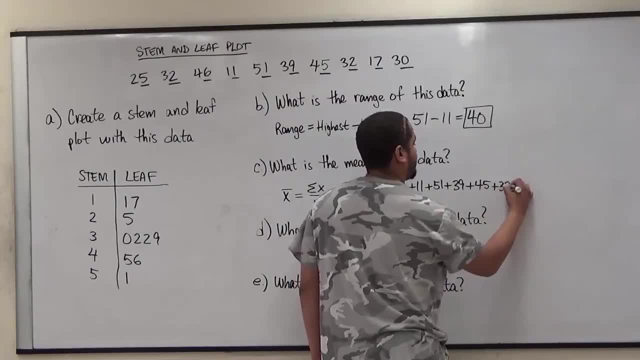 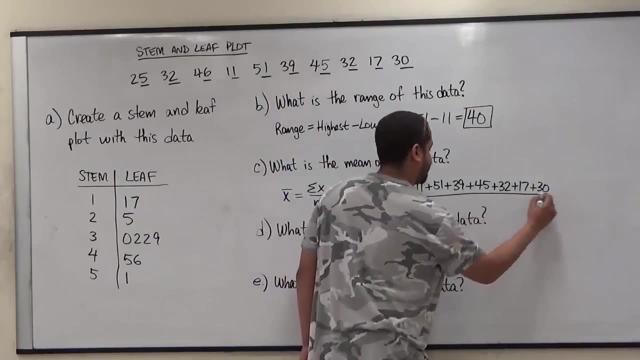 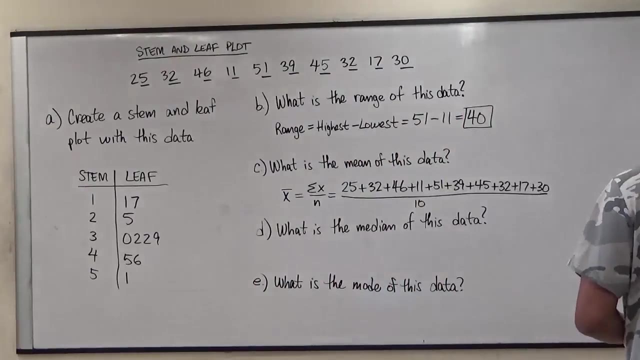 divide all of this by the number of samples we have, which I believe to be 10, right? So when we sum up these values, what we're going to get is the sum is 1,, 2,, 3,, 4,, 5,, 6,. 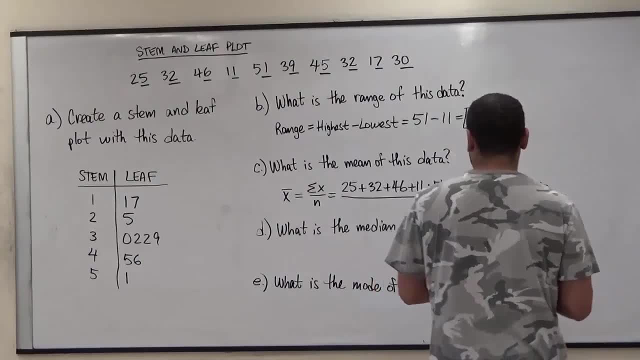 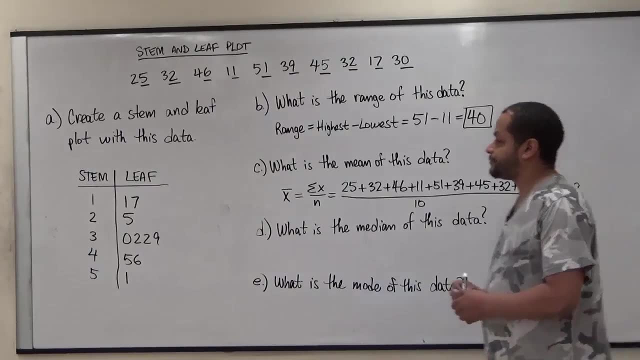 7,, 8,, 9,, 10.. We have 10 values and the sum of all these digits are going to give us 328. And we're dividing that by 10.. All right, So now, when we take the sum of these, let. 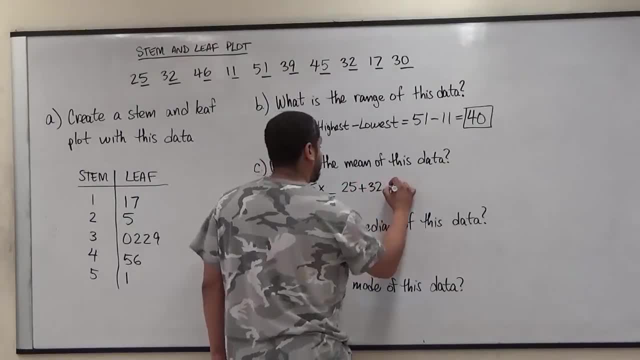 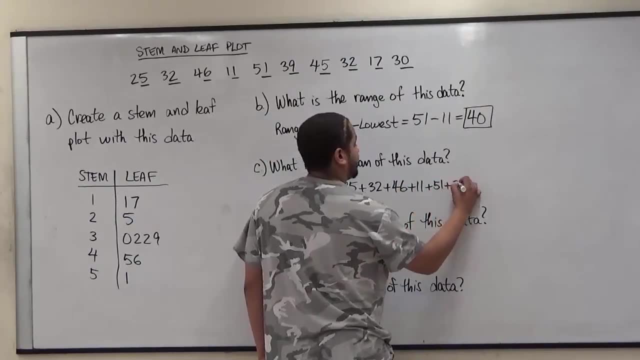 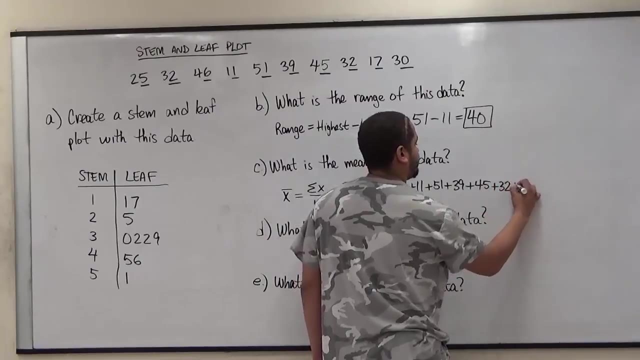 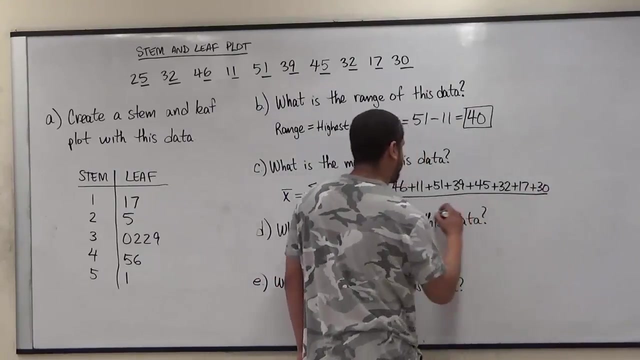 numerator. So we have 25 plus 32 plus 46 plus 11 plus 51 plus 39 plus 45 plus 32 plus 17 plus 17.. All right, plus 30. We're going to divide all of this by the number of samples we have, which I believe to be 10.. 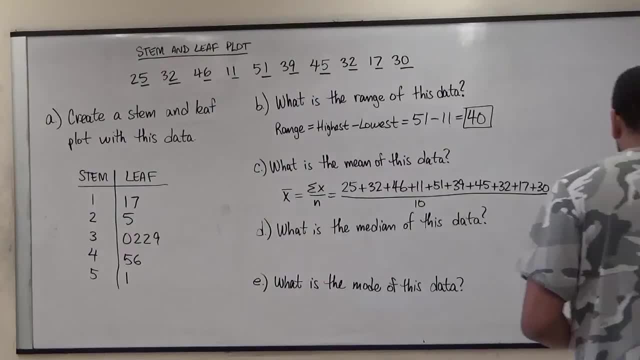 Right. so when we sum up these values, what we're going to get is: the sum is 1, 2, 3, 4, 5, 6, 7, 8, 9, 10.. We have 10 values and the sum of all these digits. 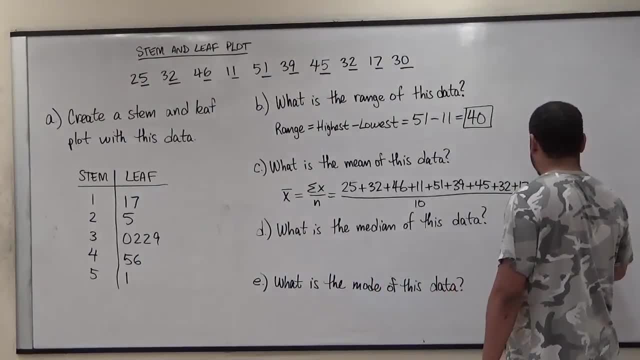 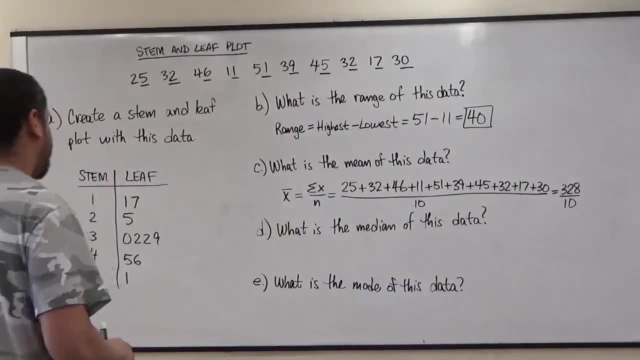 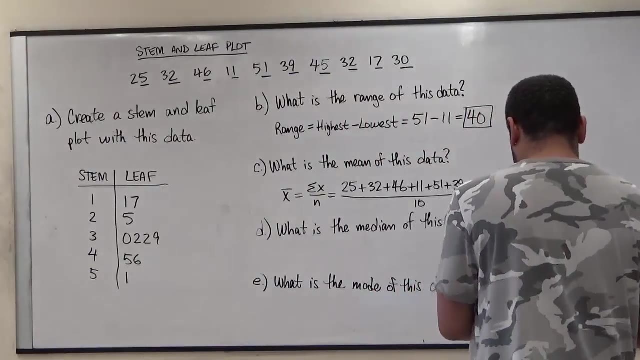 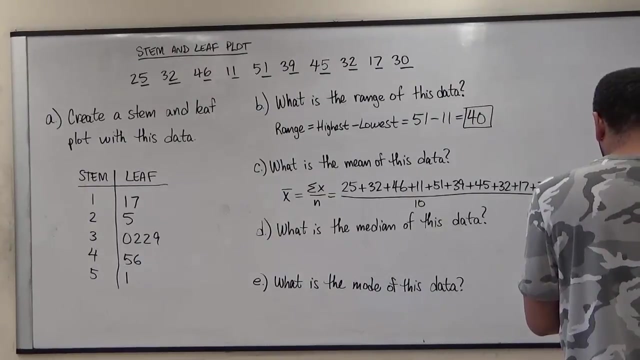 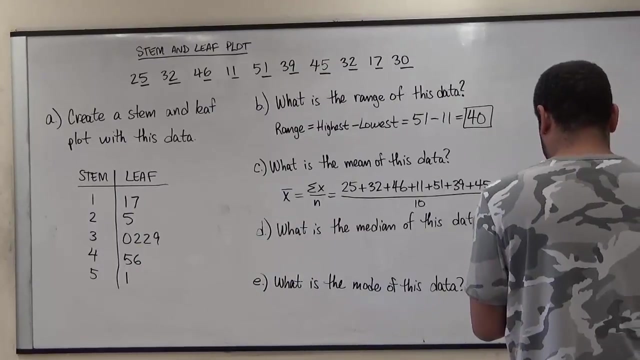 are going to give us 328.. And we're dividing that by 10.. So now when we take the sum of these, let me just double check these on a calculation to make sure our sum is correct. So we have 25 plus 32 plus 46. 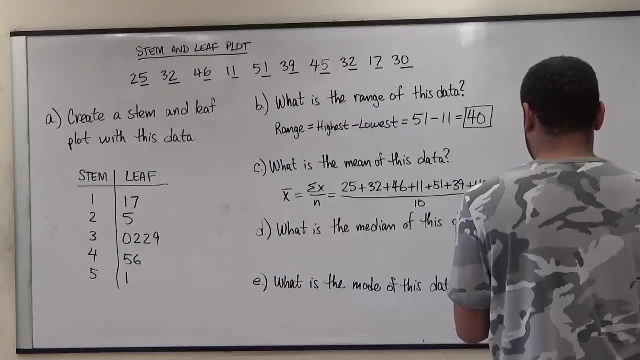 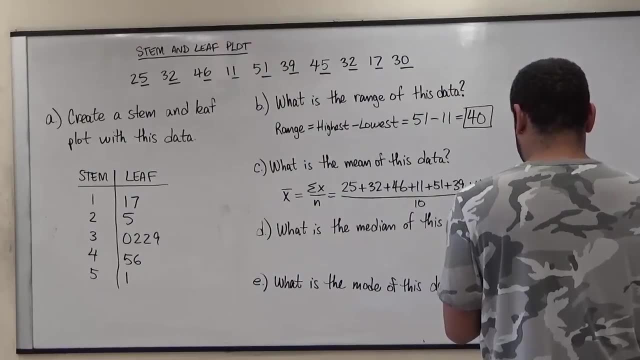 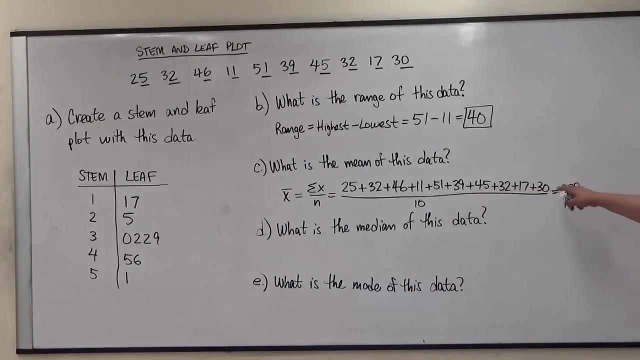 plus 11 plus 15 plus 51 plus 39 plus 45 plus 32 plus 17 plus 30. That is 328.. So now make sure you're using a calculator while adding these. Once you add them and you divide them by 10, this division is going to give us 32.8.. 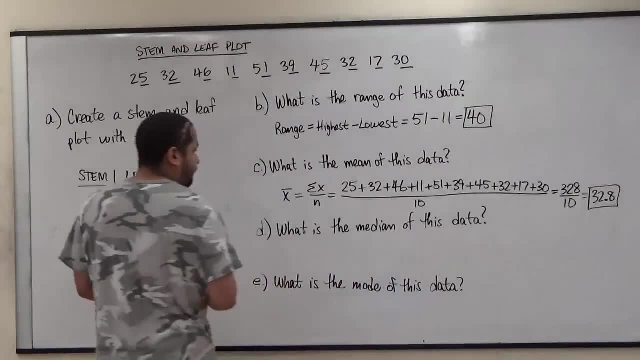 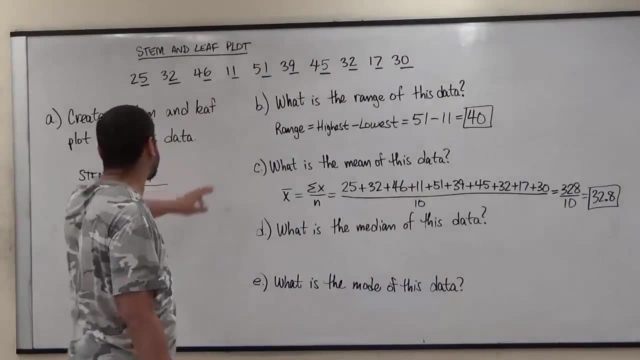 And 32.8 is our average, our mean. Following the mean, we're going to start by doing the median For median. we have to arrange the data in order, So we're going to go from lowest to highest. Instead of looking at this, to do that, we're just going to use our stem and leaf chart. 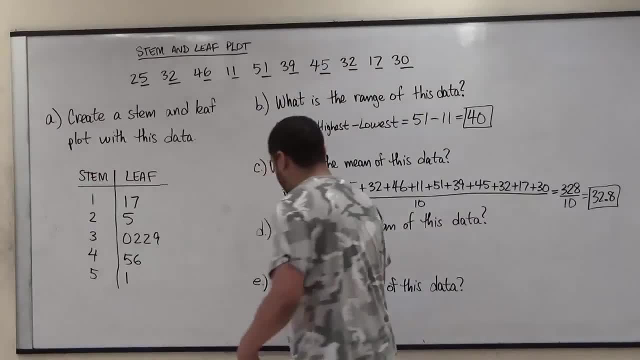 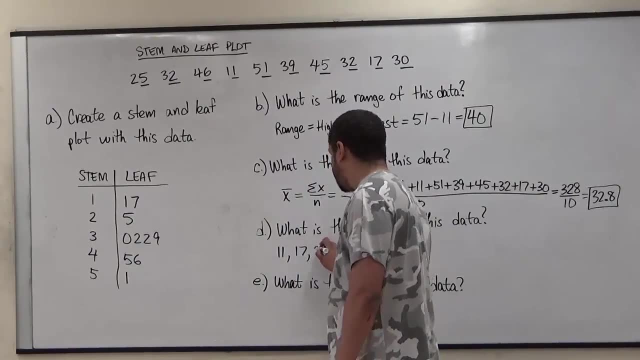 We're going to take each stem with each number and go asserting them here. So we have the first stem and leaf is 1 and 1.. The second is going to be 1 and 7.. The third, 2 and 5.. 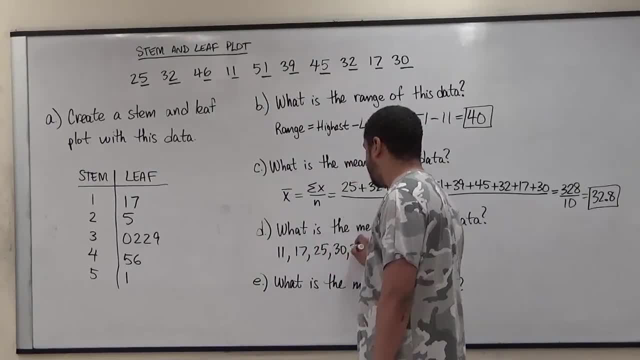 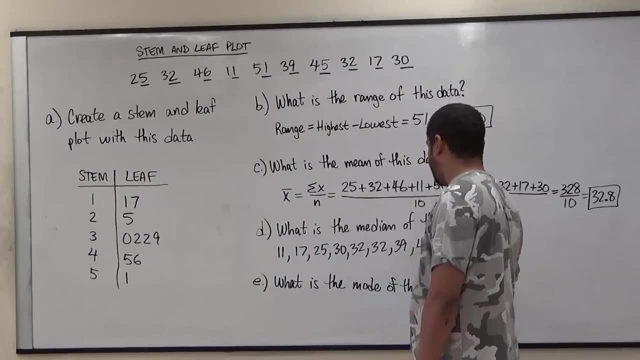 The fourth, 3, 0.. The fifth, 3, 2.. The sixth, 3, 2.. The seventh, 3, 9.. The eighth, 45.. The ninth, 46.. And the tenth is 51.. 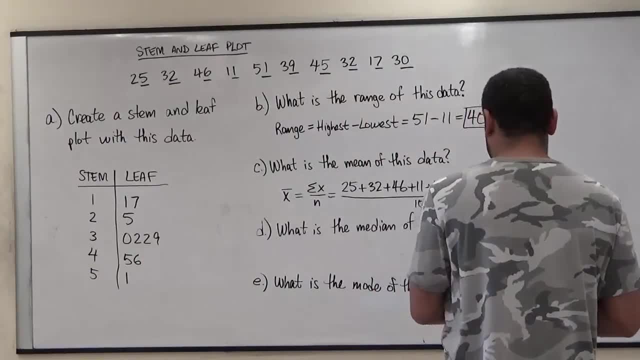 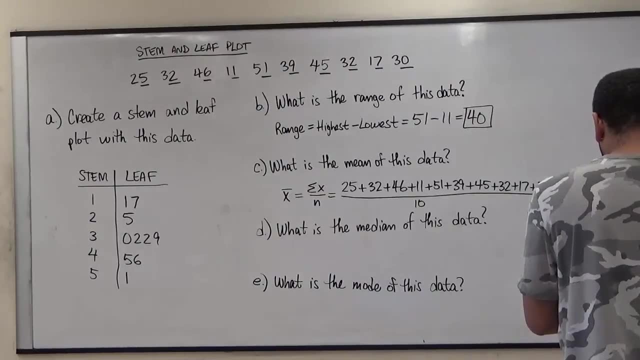 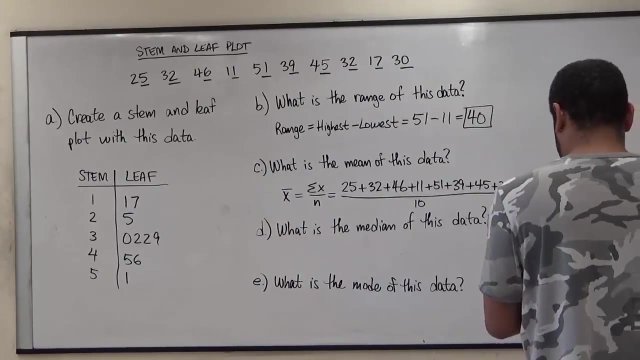 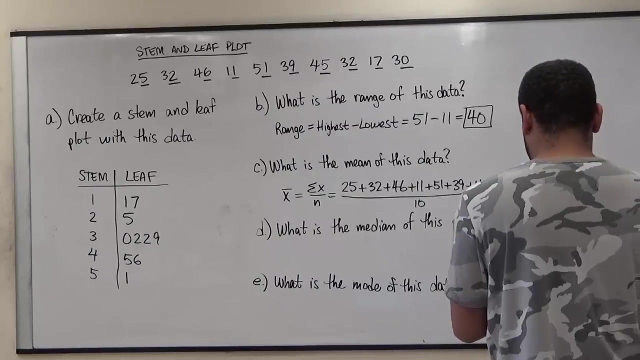 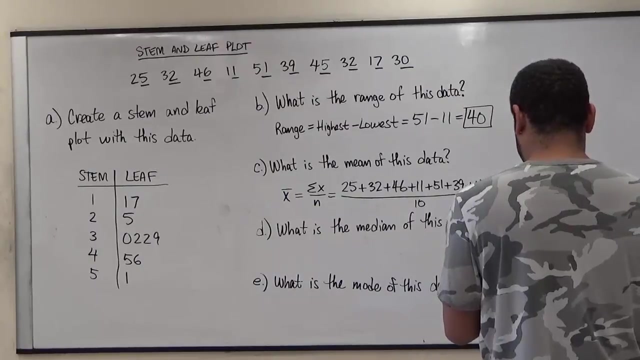 me just double check these on a calculation to make sure our sum is correct. So we have 25 plus 32 plus 46 plus 11 plus 42 plus 43 plus 42 plus 43 plus 44 plus 44 plus 51 plus 39 plus 45 plus 32 plus 17 plus 30. That is 328.. So now make sure you're. 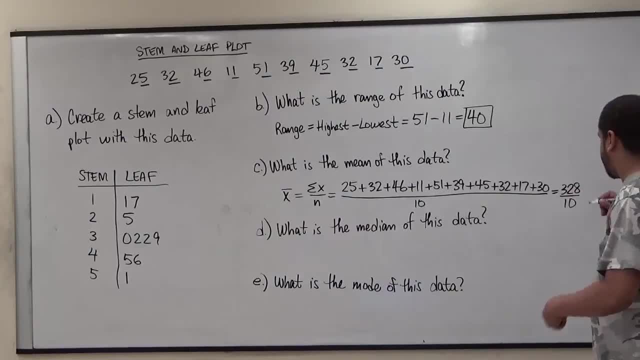 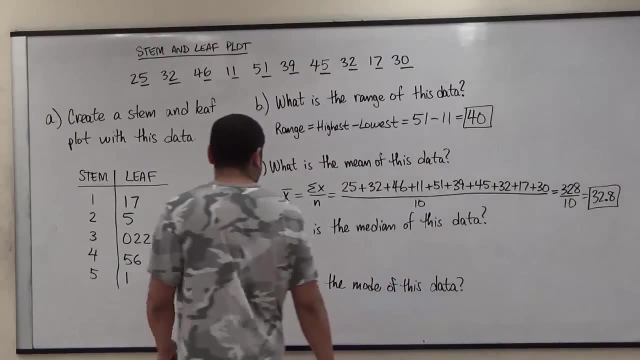 using a calculator while adding these. Once you add them and you divide them by 10,, this division is going to give us 32.8.. And 32.8 is our average, our mean. All right, Following the mean, we're going to start by doing the median. Now, to do the median, we have to 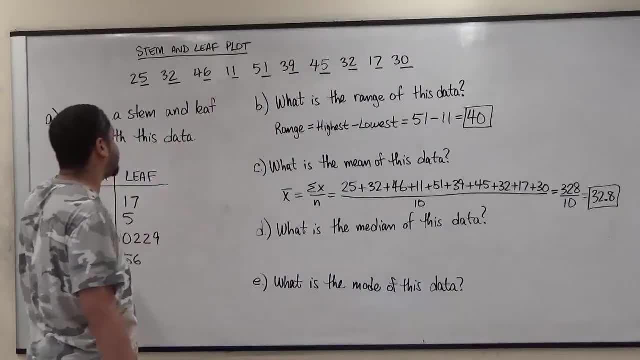 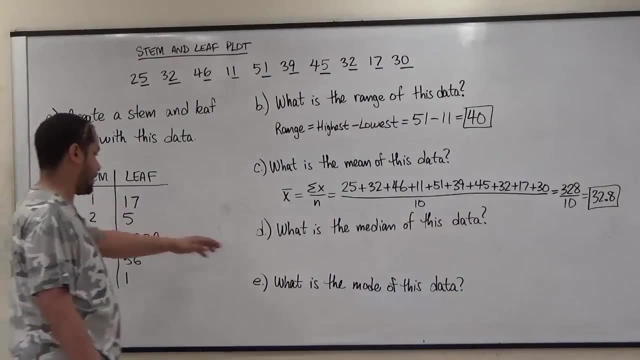 arrange the data in order, So we're going to go from lowest to highest. Instead of looking at this to do that, we're just going to use our stem and leaf chart. We're going to take each stem with each number and go asserting them here, So we have the first stem and leaf. 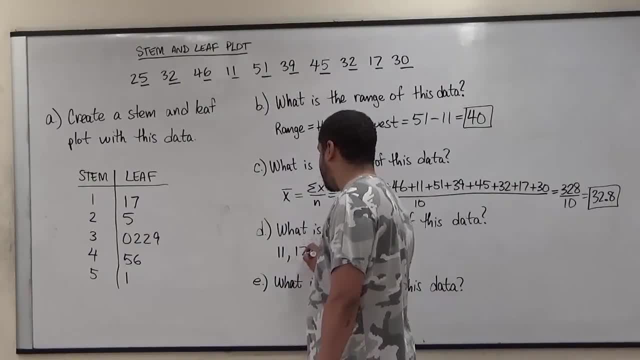 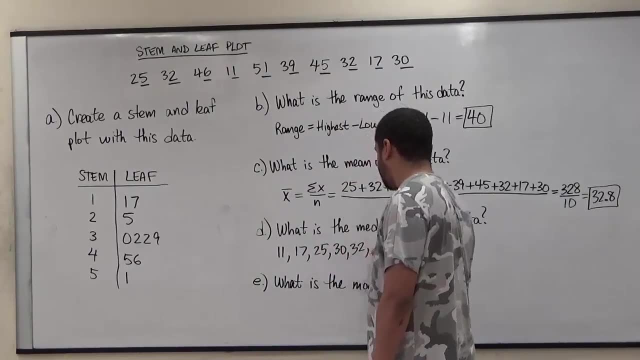 is 1 and 1.. The second is going to be 1 and 7.. The third, 2 and 5.. The fourth, 3, 0.. The fifth, 3, 2.. The sixth, 3, 2.. The seventh, 3, 9.. The eighth, 45.. The sixth, 3, 2.. The. 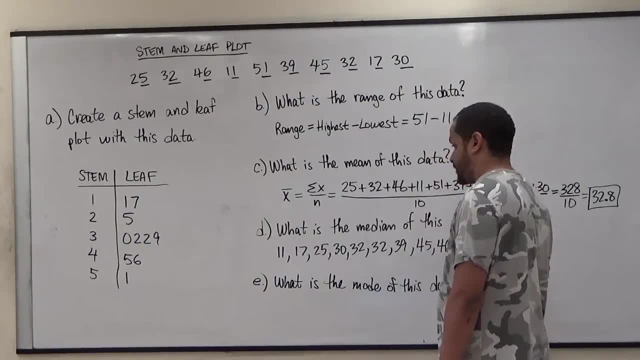 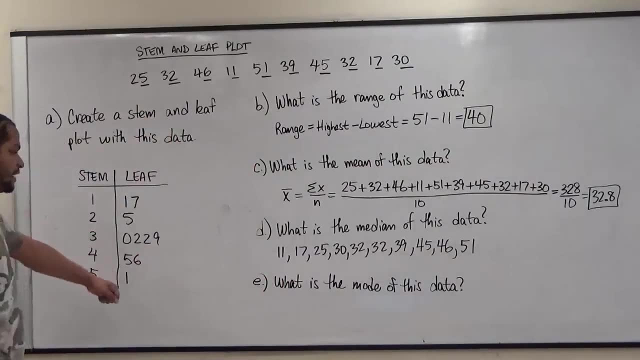 sixth, 3, 2.. The ninth, 46. And the tenth is 51.. And this is how useful a stem and leaf chart is. It helps us arrange data in order, going from smallest to highest, And what we want to do to get the median is we want to keep knocking one off of each side. 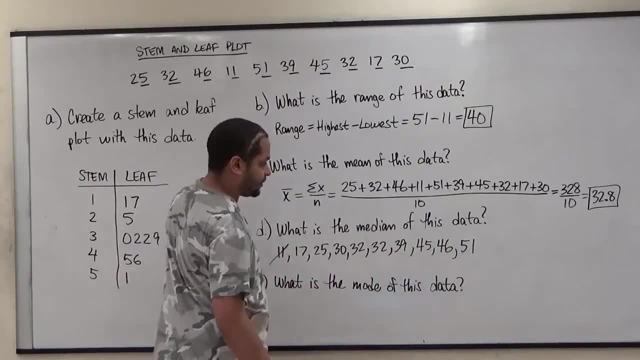 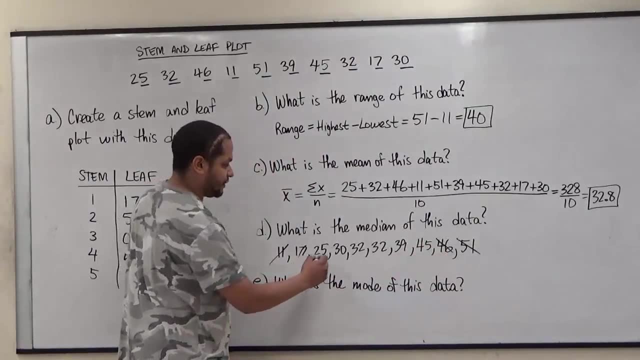 till we get to the center right. So we're going to knock off this 11 with this 51. Then we're going to knock off this 17 with this 46 and continue moving in till we close in on 2 or just 1.. 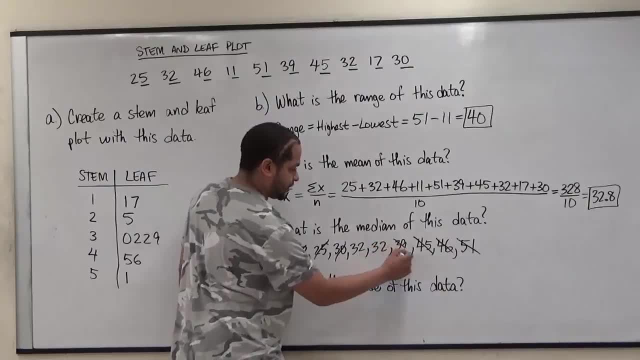 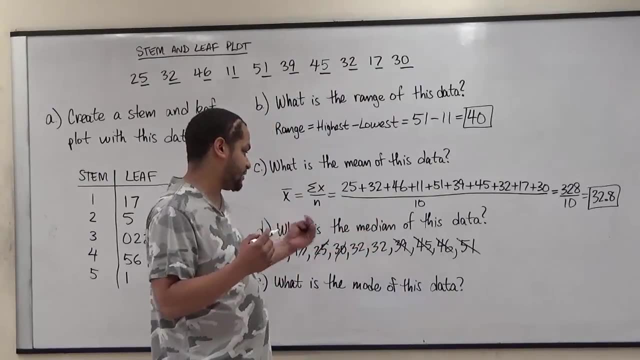 So the 25 with the 45., The 30 with the 39., And we're left with these two 32s. Now, usually, since they're the same number, we can just say the mean is the median is 32.. But what we actually have to do is: